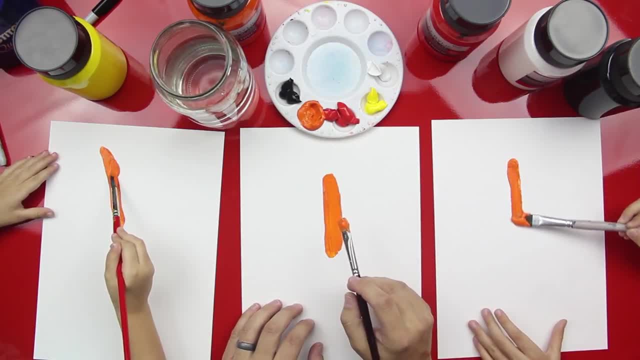 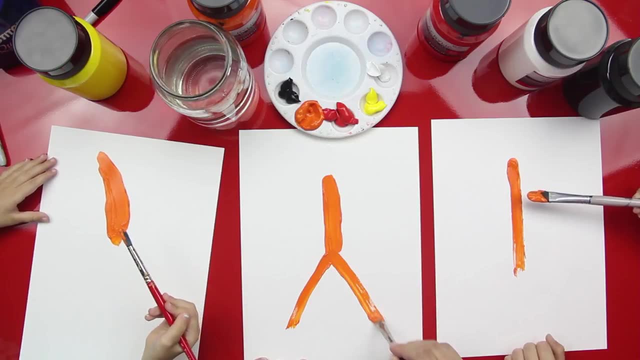 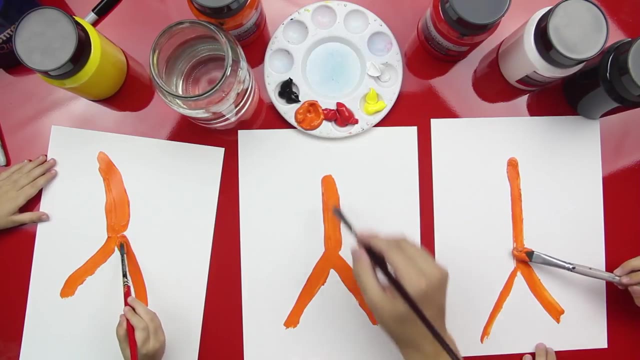 Good job Heads, Heads Checkers. You got your line Good. Okay, now we're going to do an upside down V at the bottom. Can you do an upside down V? It's like no, it's an upside down Y, An upside down Y. 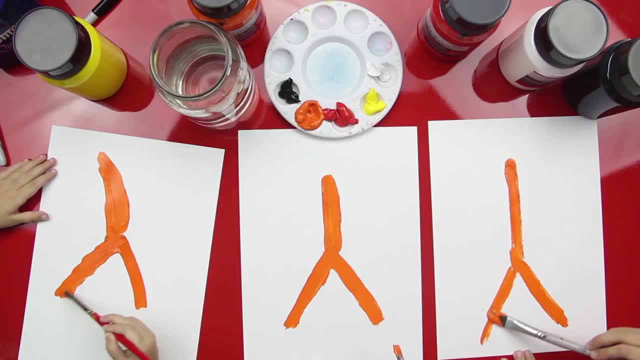 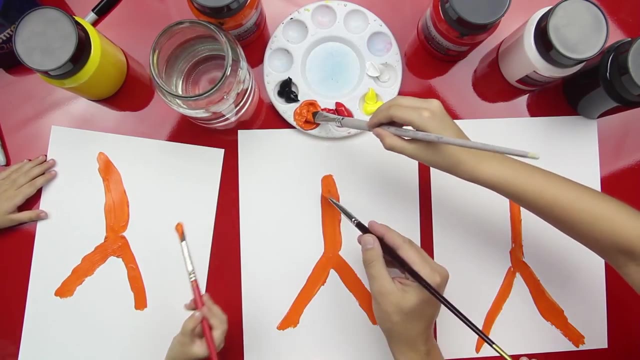 yeah, you're right. Okay, make those a little longer. Good job, Checkers, Heads- Good, And what you want to do is you want to make sure that this line is kind of the same length as those lines. Alright, okay, Now we're going to put arms on our starfish. These are its feet, this is its head, and 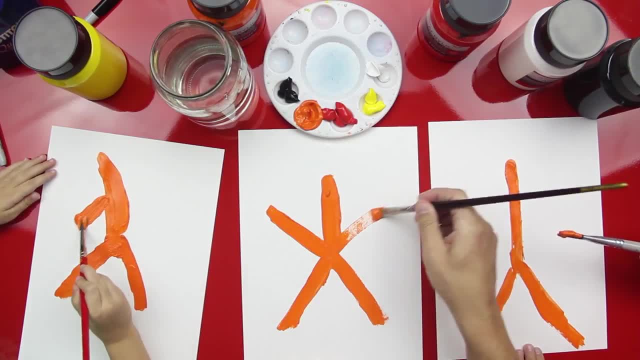 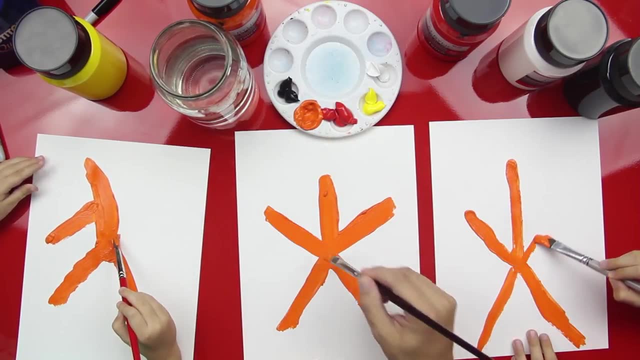 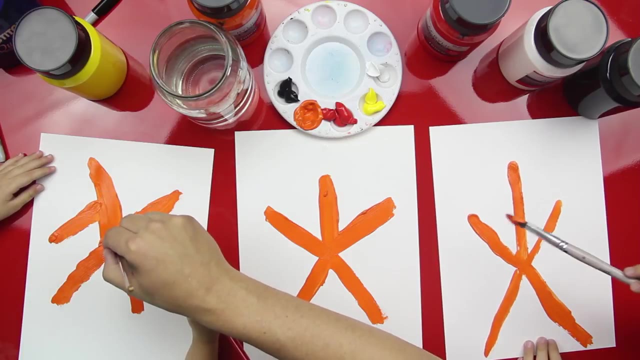 this is its arms, So do a little line that comes out for the arms, like that: Good job Heads. Oh, and then this one, this one. you kind of want it to come out of the middle. See, this is the middle, and so you want this to come out and go up. You want to go ahead and try that, So you draw a nice. 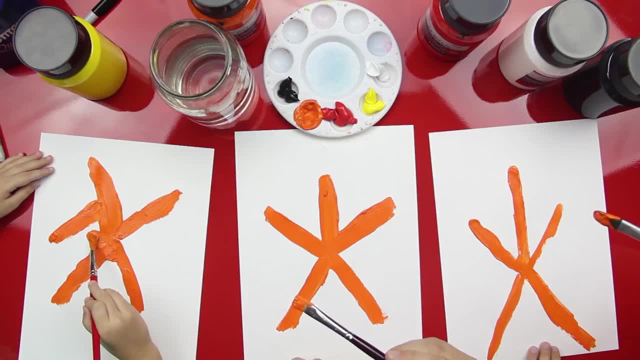 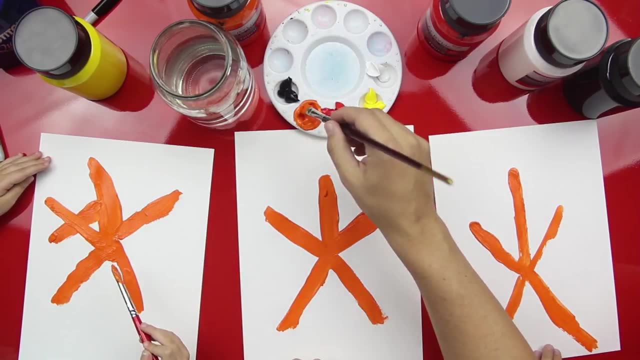 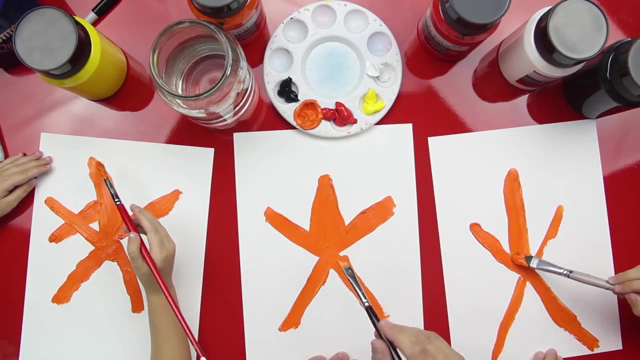 line going this way. there you go, yes, and we will go all the way over here. good job, and then we'll. I'll show you, we'll cover that up. okay, now up here at the top we're gonna make kind of a triangle shape. see how we turn that head into a. 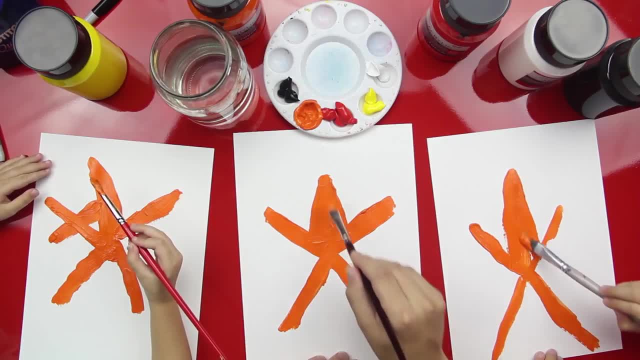 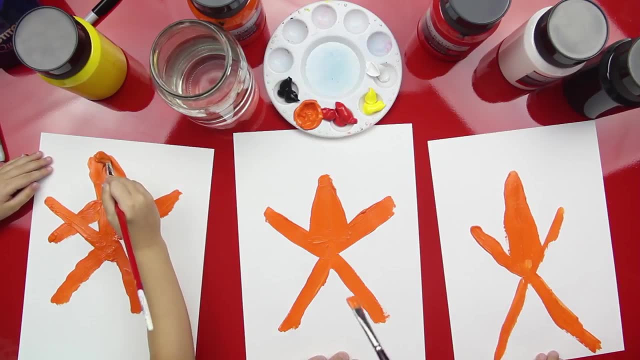 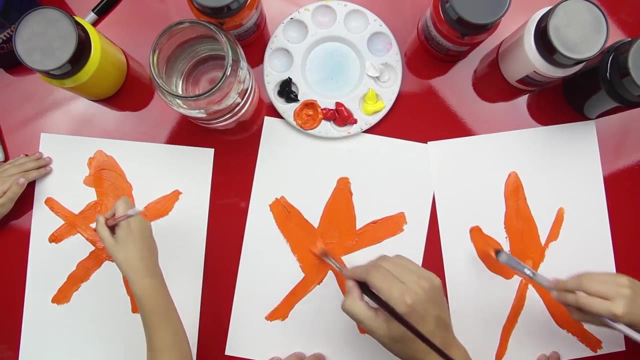 kind of a triangle. so you look at the triangle. you see that hats. can you try that? good job checkers, good job heads. all right, now we're gonna do it to this one. what's this? turn it into a triangle, all right, all right, good, then we're. 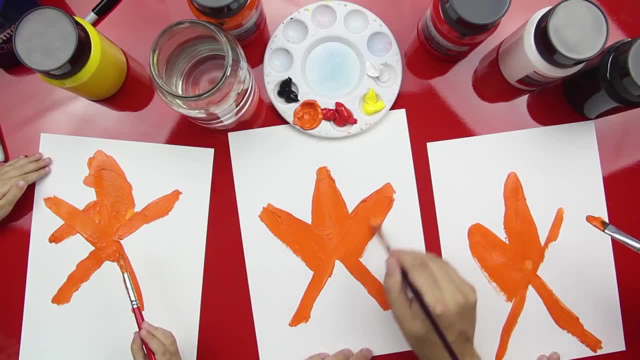 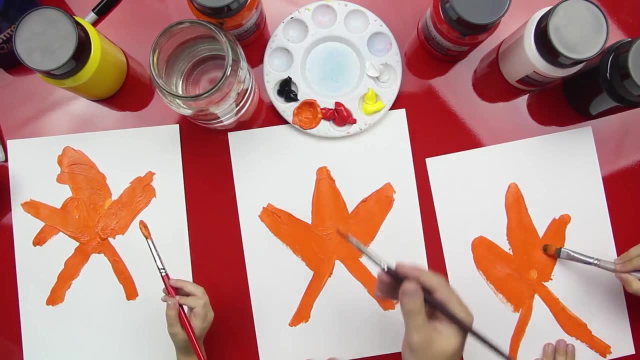 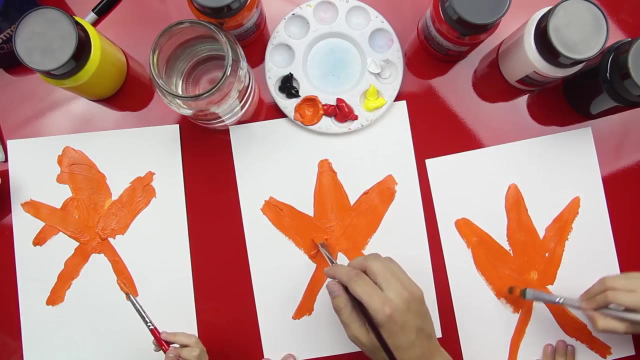 gonna turn this one into a triangle. you do that, okay, a little more good job checkers. you can make this one a little bit longer. there you go. and then truckers wanted to do this one, even though this one's kind of an easy one. he just wanted to have fun. huh yeah, and 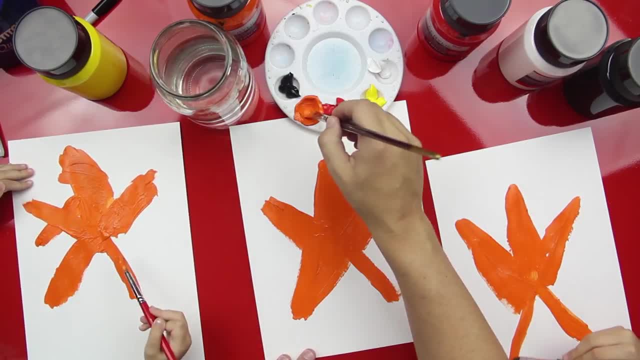 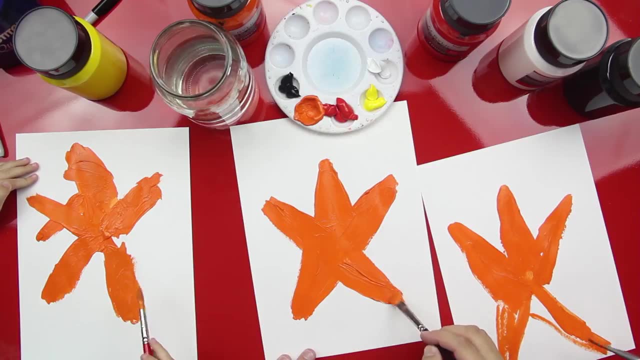 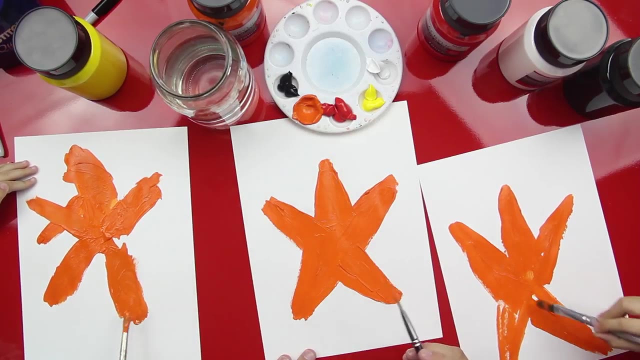 there's nothing wrong with that. okay, I'm making this one bigger. now I'm gonna make this one bigger. good job, heads. you want little points on the end? see this. see how there's a little point on the end. I love acrylics, so this smell kind of. 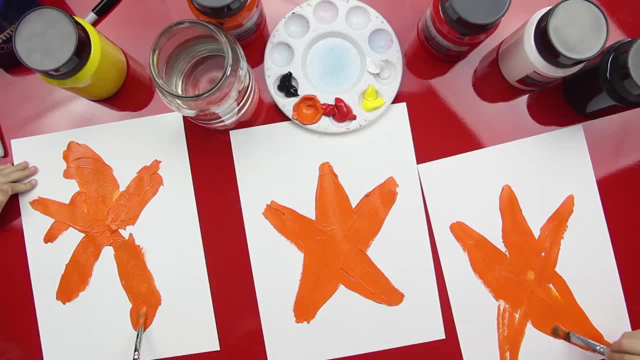 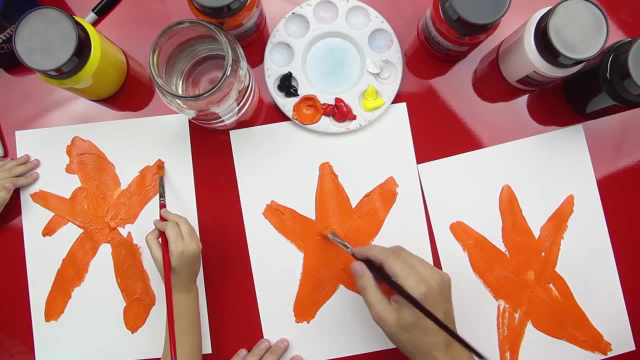 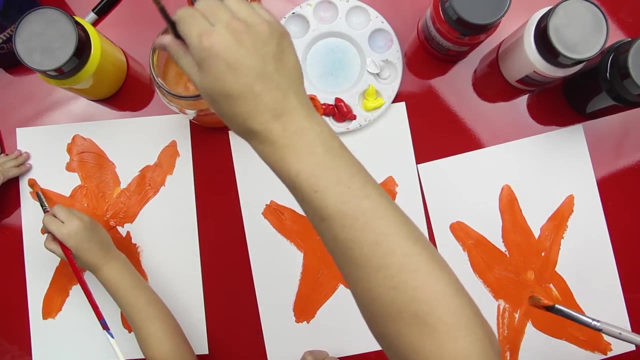 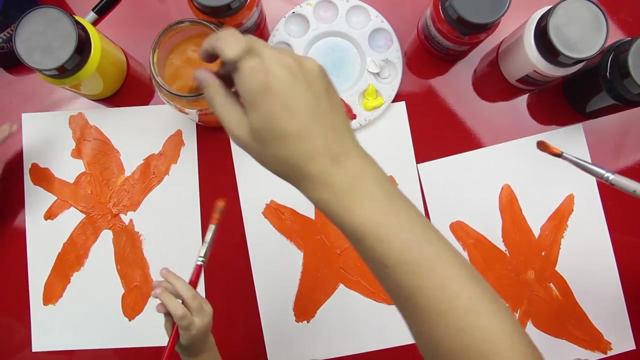 strong, huh, so had to do a little point. there you go. it does kind of look like orange, Patrick, all right. okay, now let's rinse off. let's rinse off your paintbrush. is that a lot of orange in there? did you get a little point on each? on each of your arms? okay, why is it? why are we doing a starfish? we? 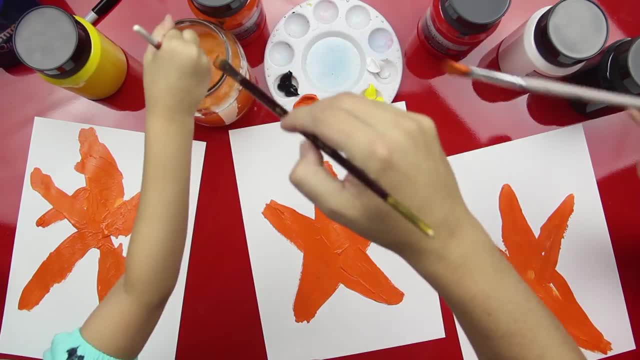 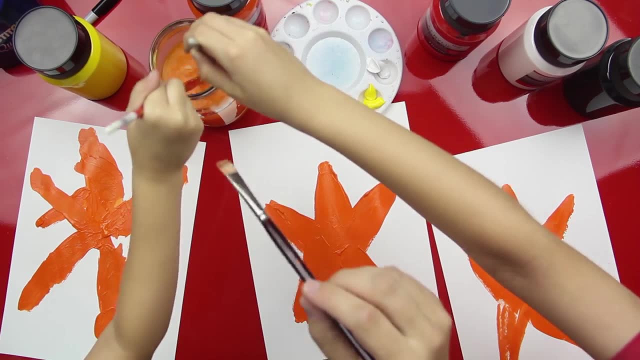 do you know what's special about this week? super cool, it's Shark Week, so we're doing it. they have a show on TV where they talk about sharks all week long. okay, here you go, you can draw, you can kind of wipe it off a little bit, and 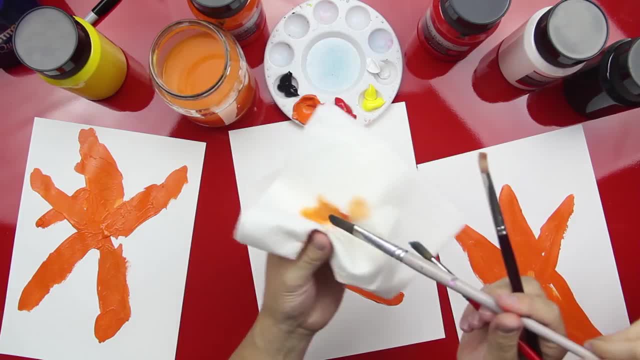 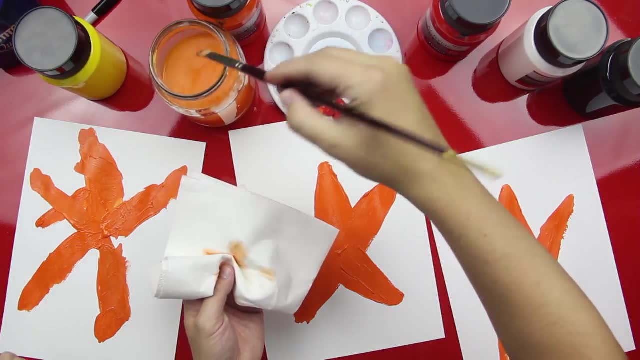 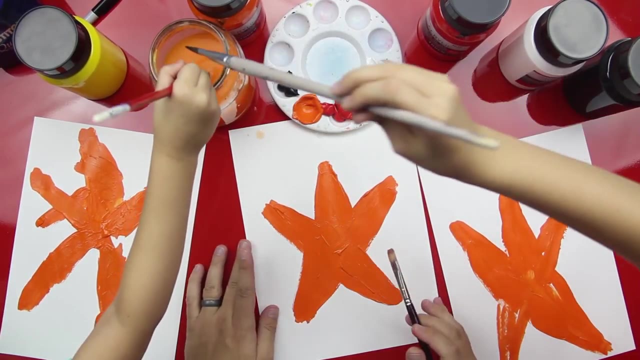 so we thought it would be fun this week to do everything that has to do with the ocean, that cool. that's why we're doing a starfish, all right, okay, ready for? okay, get a little water on there now, just a little bit, and then we're gonna do a. 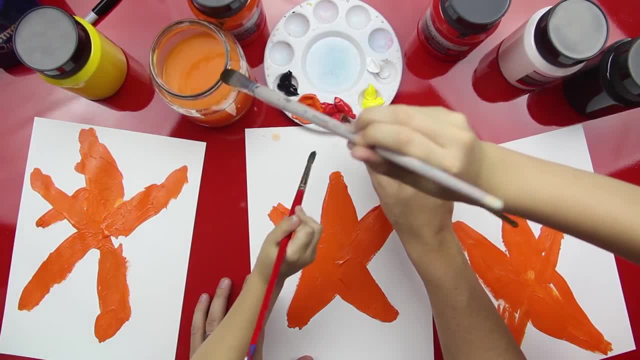 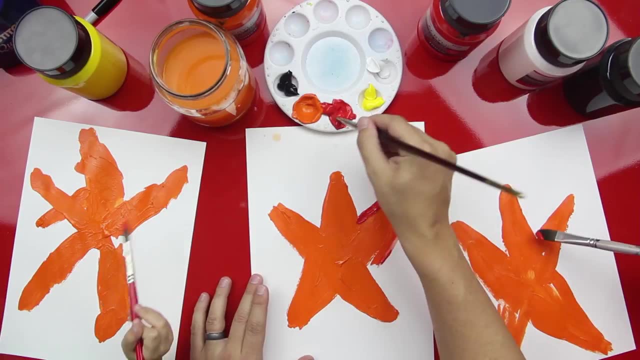 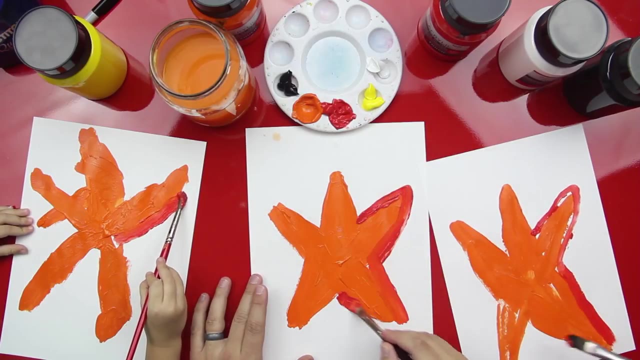 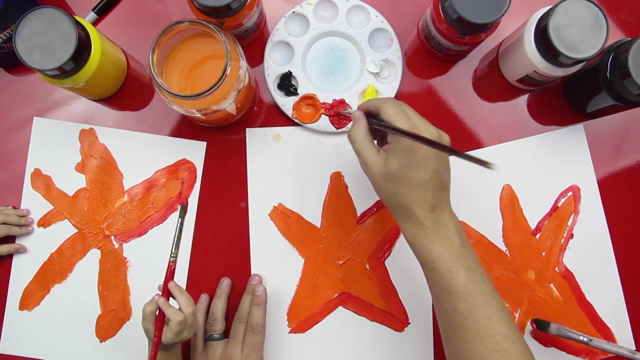 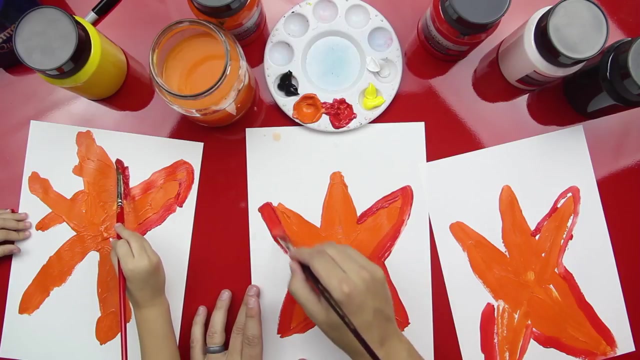 red and what we do with the red is we're gonna go around the outside of the red, outside the orange, and trace it with the red. this is kind of gonna make the outside of the starfish look a little darker and it might even blend, and that's okay. if it blends, how's this looking? awesome and for our art friends. 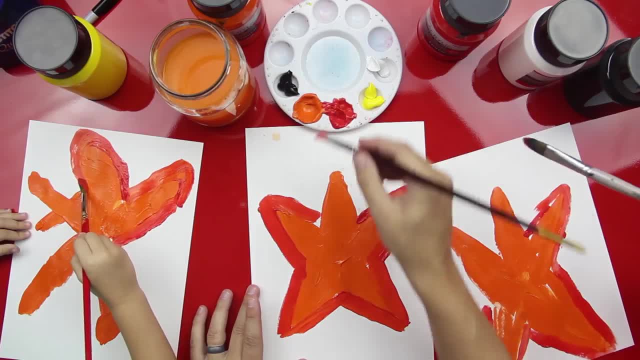 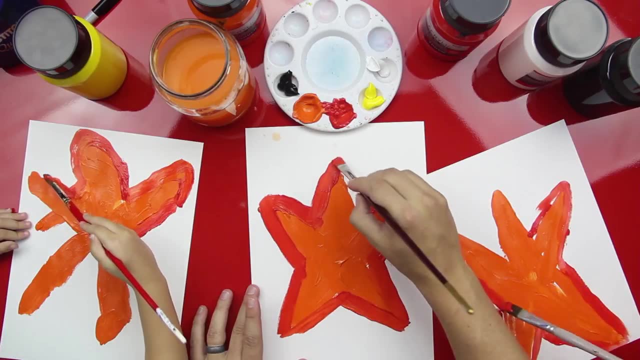 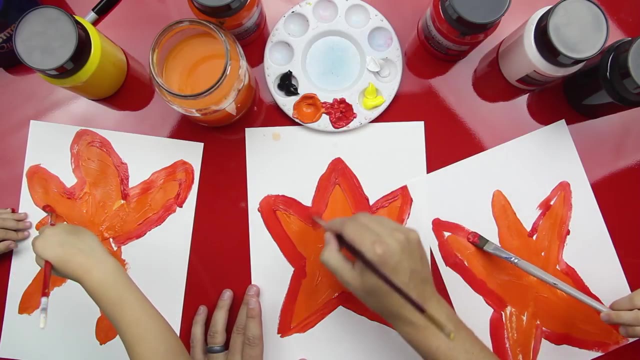 at home if your parents are a little worried about you getting messy. yeah, we're doing this art project. you guys can get an old shirt. you can put an old shirt on. get one of your dad's old shirts- preferably not one of his good shirts, one of his old shirts. save them. he's gonna throw some shirts away. make. 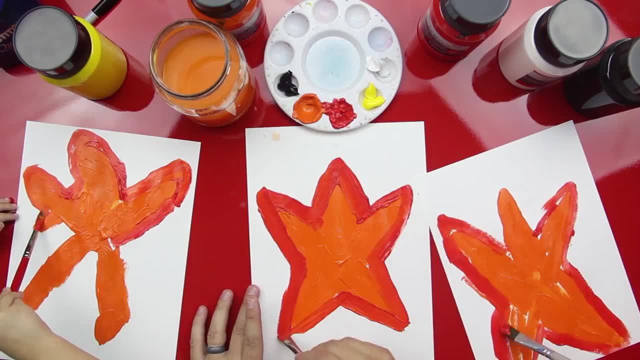 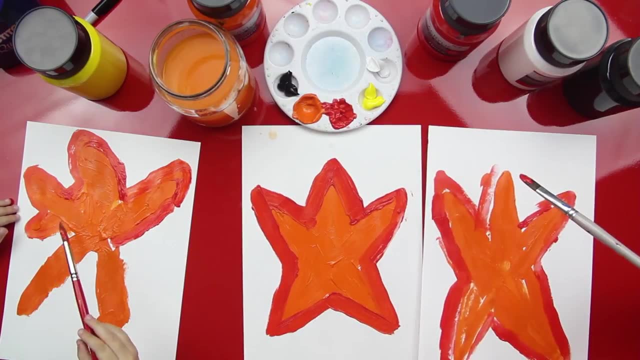 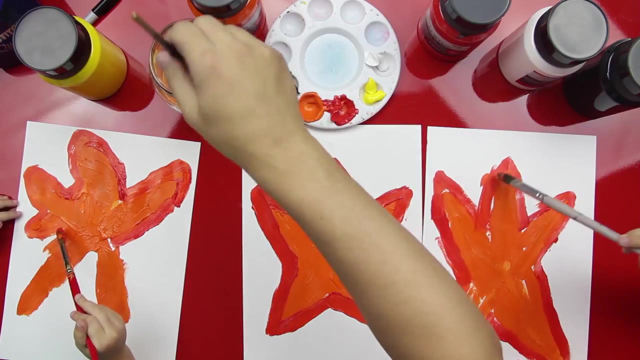 sure to throw some shirts away. and throw some shirts away and throw some shirts away, to grab them and say, hey, dad or mom, can I have your old shirt and then save it. hey, get your painting off, my painting, you silly. all right, you guys got your red all the way around. keep going heads and then you guys can use those old 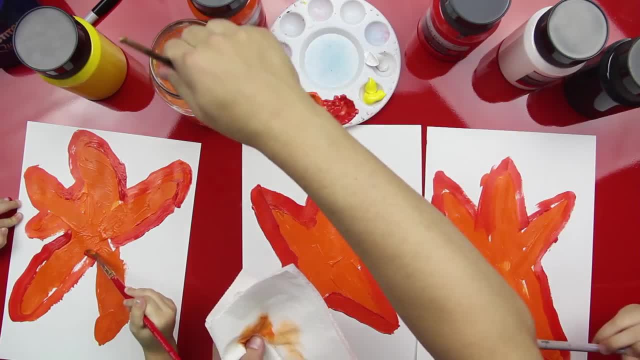 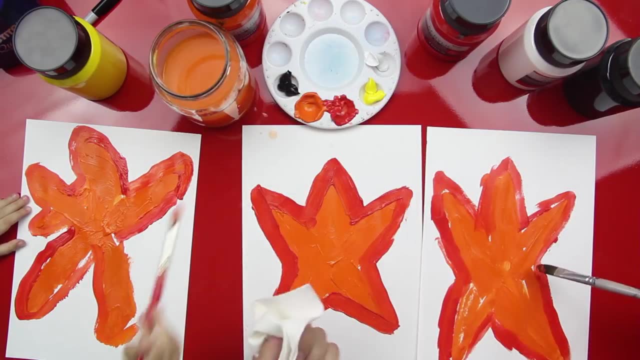 shirts and that will protect your nice shirts from getting paint on them. so if you get a little paint on your old, on your dad's old shirt, it's okay. it's called a paint job, a picture picture. yeah, good job heads. you're almost done. you're making a. 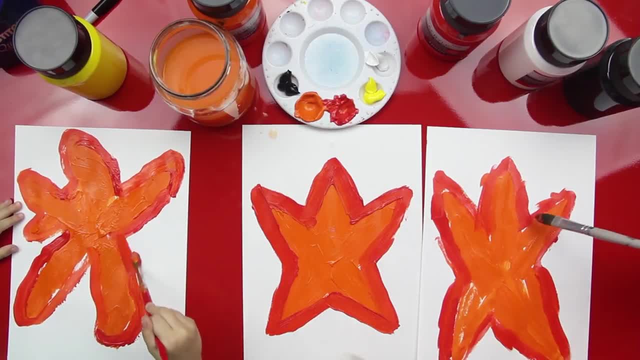 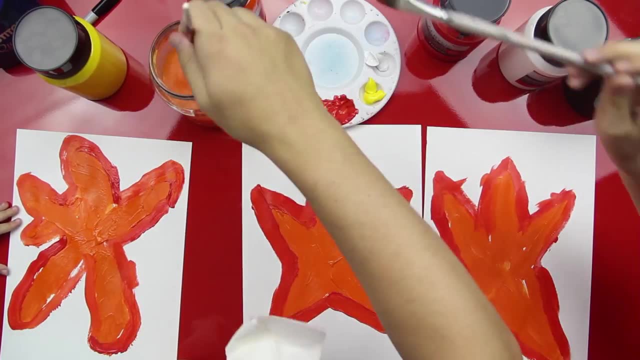 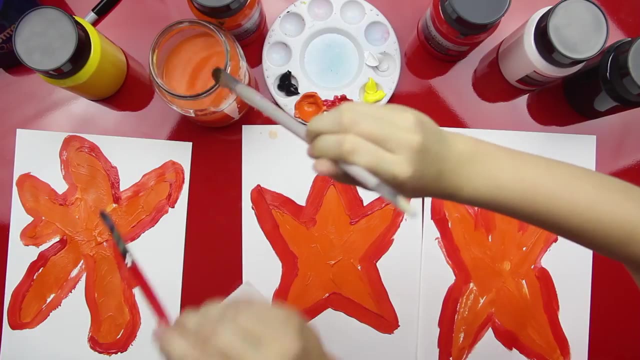 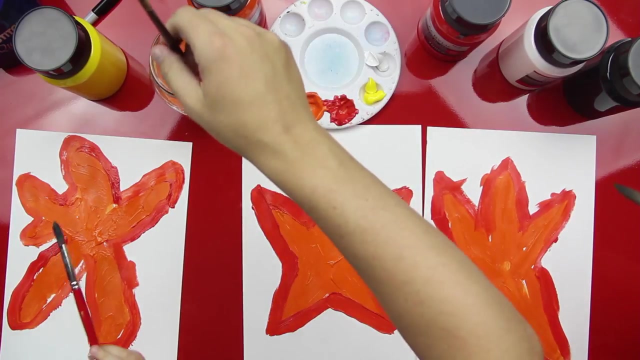 little better. you can fill in the little red right there. there you go. good job, get that paint off. okay, ready for the next one. yeah, okay, next color, we are gonna do yellow. a little water on there? okay, here you go, hats checkers. okay, here you go, hats checkers. okay, all right, you'll get a little yellow on. 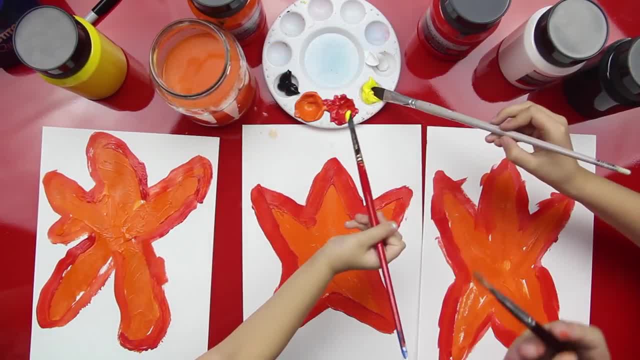 okay, all right, you'll get a little yellow on our paintbrush. make sure you have you our paintbrush. make sure you have you our paintbrush. make sure you have you. saw some water? good, okay, watch this we're. saw some water- good okay, watch this we're. 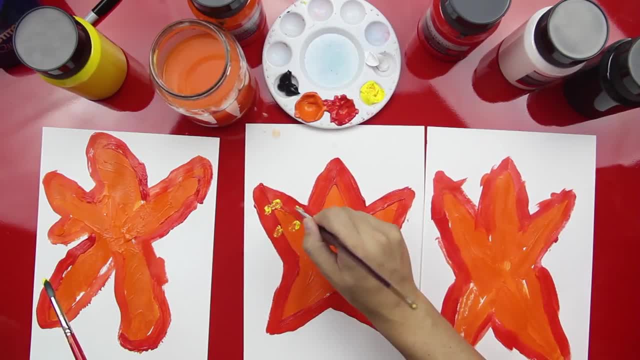 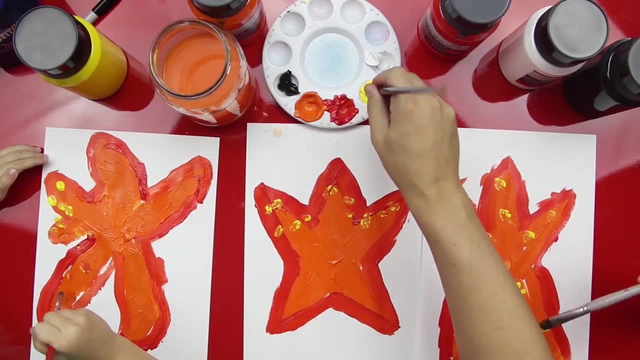 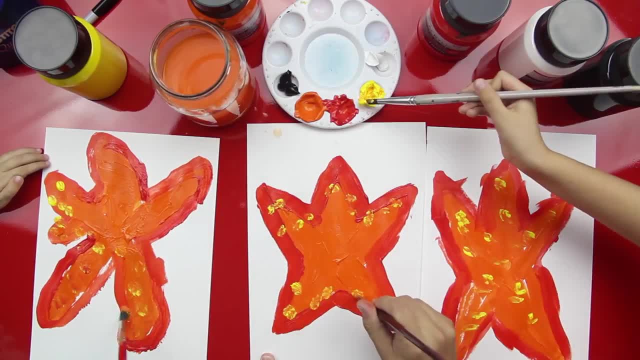 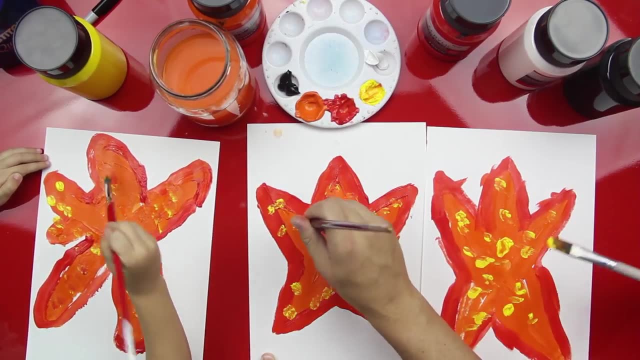 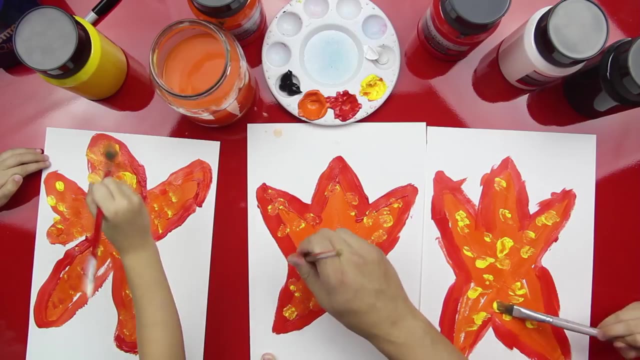 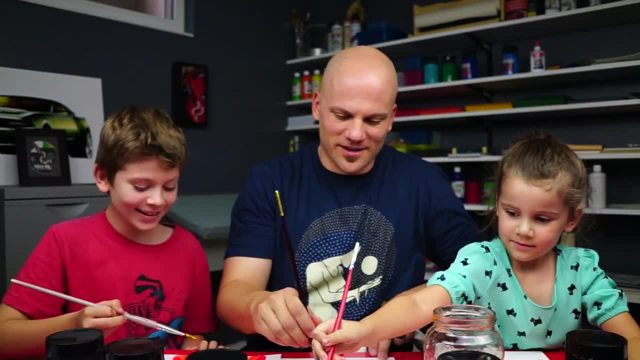 look at it, she's doing awesome. oh, she's. look at it, she's doing awesome. oh, she's going out of control. going out of control, going out of control. careful you don't get oh checkers, just careful you don't get oh checkers, just careful you don't get oh checkers, just got my arm. 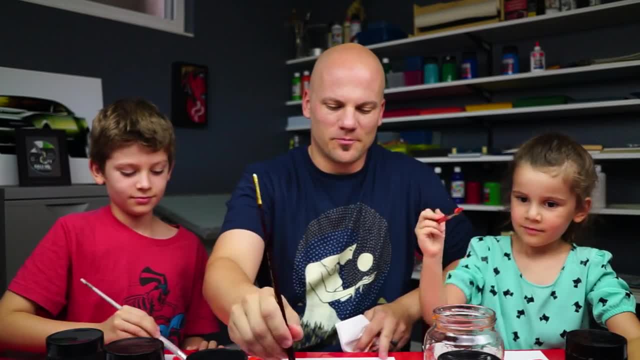 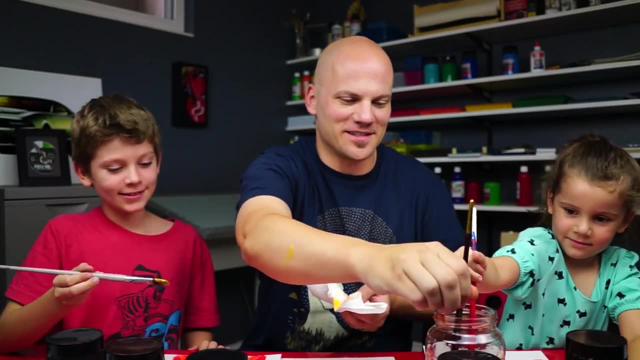 got my arm, got my arm. all right, good, okay. all right, good, okay. all right, good, okay, let's rinse off that. let's rinse off that, let's rinse off that, and then we're gonna do white, and then we're gonna do white, and then we're gonna do white for the eyes. 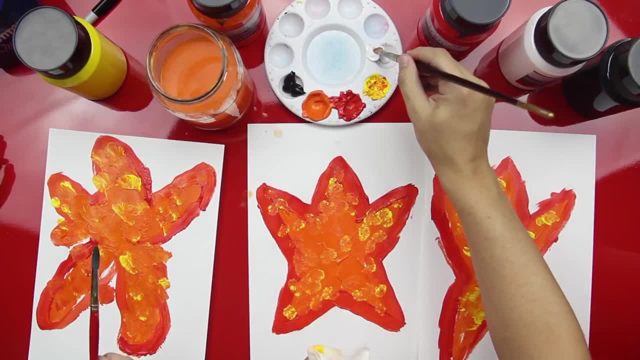 for the eyes. for the eyes: okay, you ready, we're gonna do. okay, you ready, we're gonna do. okay, you ready, we're gonna do. we're gonna do white now, and this is we're gonna do white now, and this is we're gonna do white now, and this is gonna be for the eyes, and i kind of got. 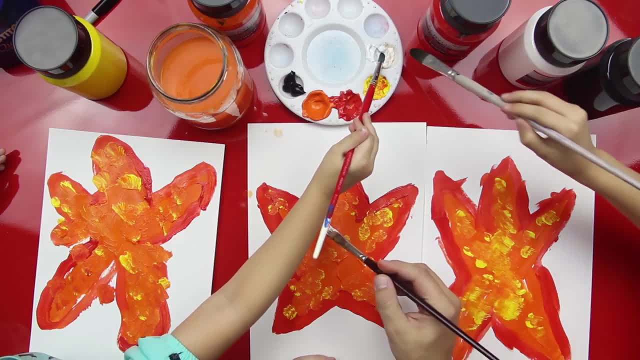 gonna be for the eyes and i kind of got gonna be for the eyes and i kind of got all the all the all the orange out of my paintbrush myself, a orange out of my paintbrush myself, a orange out of my paintbrush myself a little bit. so we're gonna do. 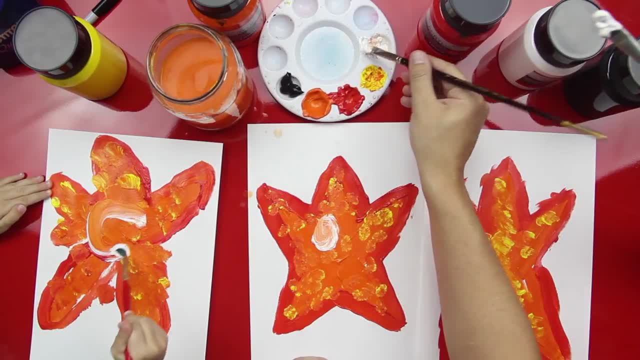 little bit, so we're gonna do little bit, so we're gonna do. we're gonna do big white, that's all right. we're gonna do big white, that's all right. we're gonna do big white, that's all right. okay, do big white. oh, heads, try and keep. 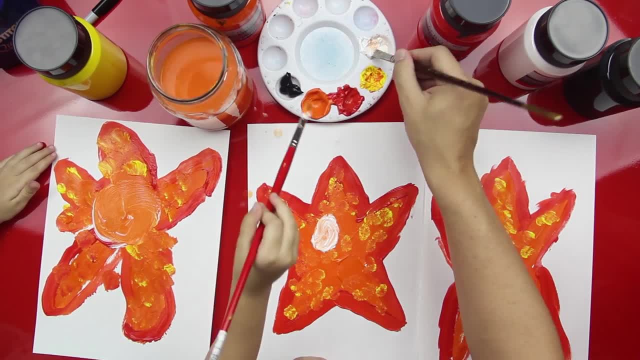 okay, do big white, oh heads, try and keep. okay, do big white, oh heads, try and keep it it it. try and keep it white. you're gonna, you're mixing it. try and keep it white. you're gonna. you're mixing it. try and keep it white. you're gonna. you're mixing it, that's okay. 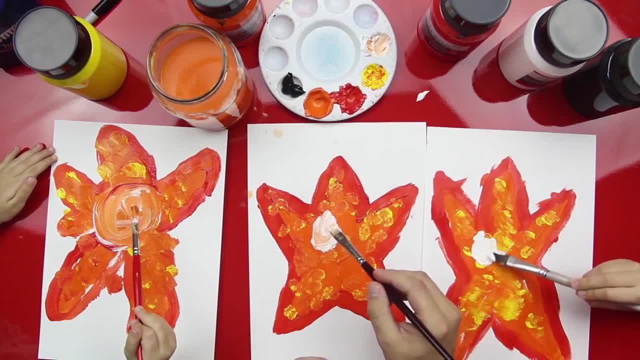 that's okay. that's okay, keep going. do a little white look heads, keep going. do a little white look heads, keep going. do a little white look heads like a little circle for the eye and like a little circle for the eye and like a little circle for the eye, and then i'm gonna do another little circle. 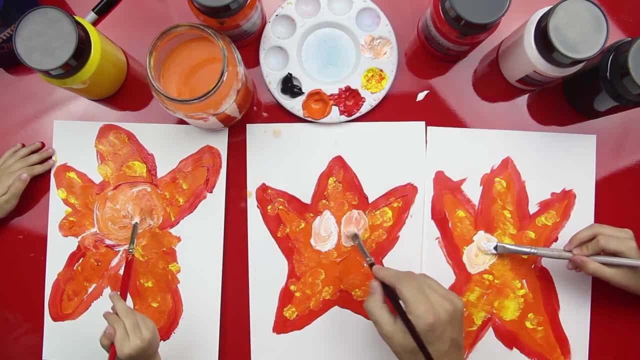 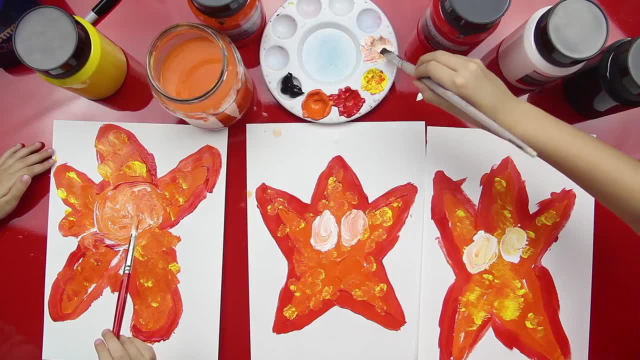 then i'm gonna do another little circle, then i'm gonna do another little circle for the other eye, for the other eye. okay, we're gonna do black, and i just okay, we're gonna do black, and i just okay, we're gonna do black and i just wipe mine off. 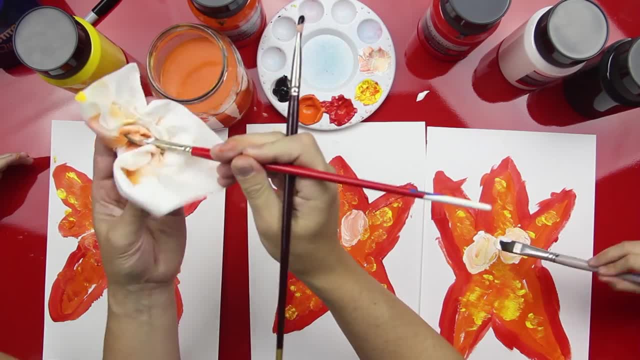 wipe mine off. wipe mine off. you go heads, i'll wipe yours off you. can you go heads, i'll wipe yours off you. can you go heads, i'll wipe yours off. you can get some black. get some black, get some black. good job, little girl doing awesome. 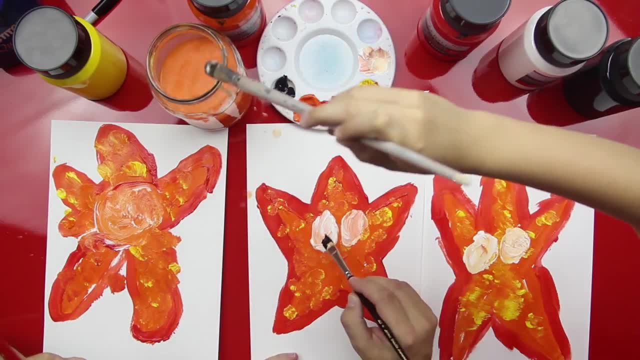 she got a little excited about making a. she got a little excited about making a. she got a little excited about making a big circle, big circle, big circle. all right, okay, now i'm gonna do a big eye. all right, okay, now i'm gonna do a big eye. 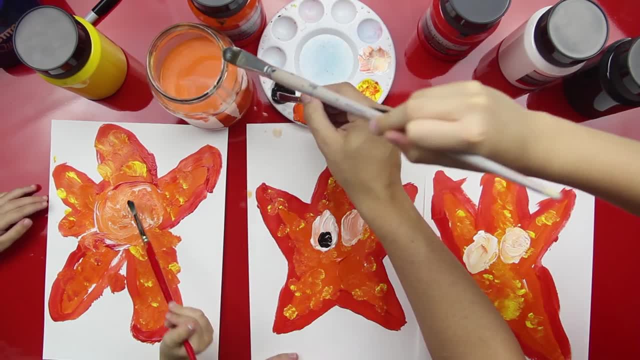 all right. okay, now i'm gonna do a big eye right in the middle, right in the middle, right in the middle, and do it. i'm gonna do another one right and do it. i'm gonna do another one right and do it. i'm gonna do another one right here. you're gonna do a big eye heads. 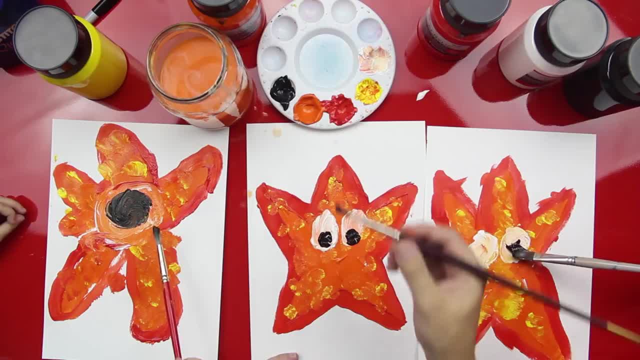 here you're gonna do a big eye heads. here you're gonna do a big eye heads, one big eye. i like it, one big eye, i like it, one big eye, i like it, and then i'm gonna do a big smile, right, and then i'm gonna do a big smile right. 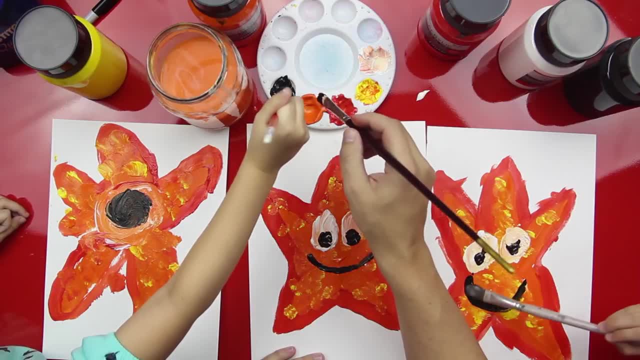 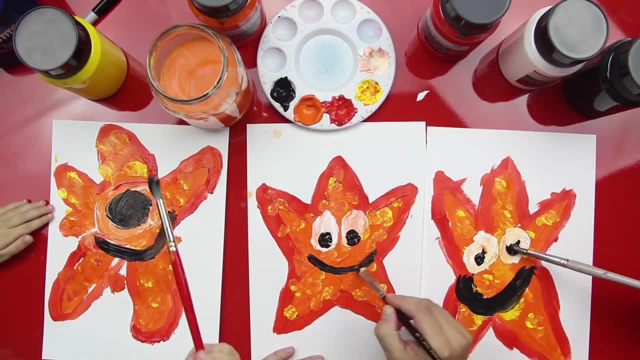 and then i'm gonna do a big smile right here here, here, you're gonna do the big smile, you're gonna do the big smile, you're gonna do the big smile. good job heads, good job heads, good job heads. whoa, that's awesome checkers. whoa, that's awesome checkers. 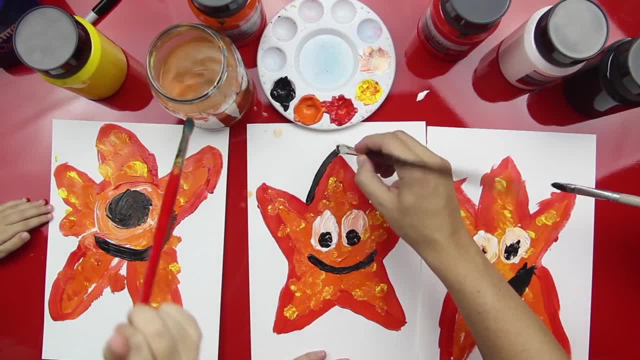 whoa, that's awesome checkers. you know what else we could do. we could you know what else we could do. we could you know what else we could do. we could do this black. we could do the black that. do this black. we could do the black that. 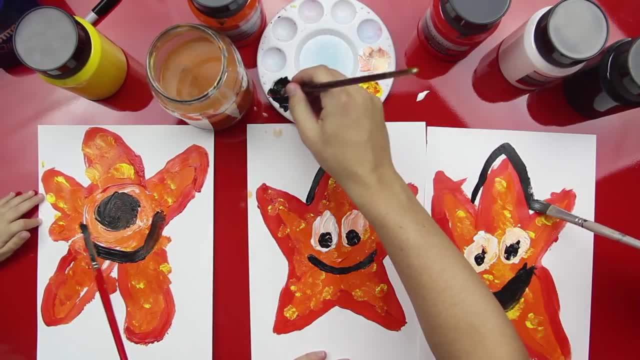 do this black. we could do the black that goes over and around and trace the goes over and around, and trace the goes over and around and trace the outside of the starfish. yeah, i'm going to scoot your paper over. yeah, i'm going to scoot your paper over. 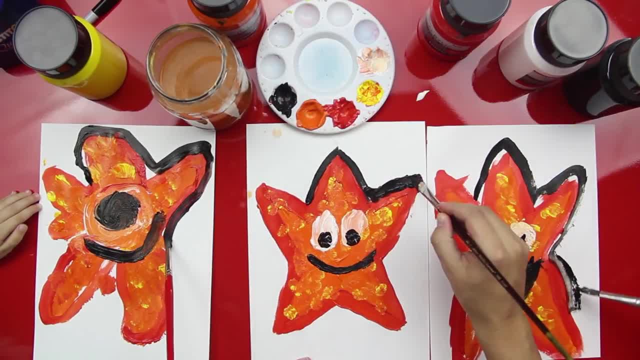 yeah, i'm going to scoot your paper over a little bit, a little bit, a little bit. yeah, hats, that's perfect. look at that. yeah, hats, that's perfect, look at that. yeah, hats, that's perfect, look at that. i like how that looks. i like how that looks. 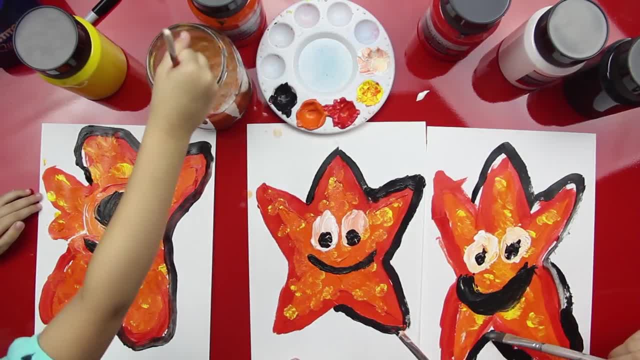 i like how that looks. you know we got some red, that's okay. you know we got some red, that's okay. you know we got some red, that's okay. oh, now it's brown brown. oh, you're mixing. oh, now it's brown brown, oh, you're mixing.